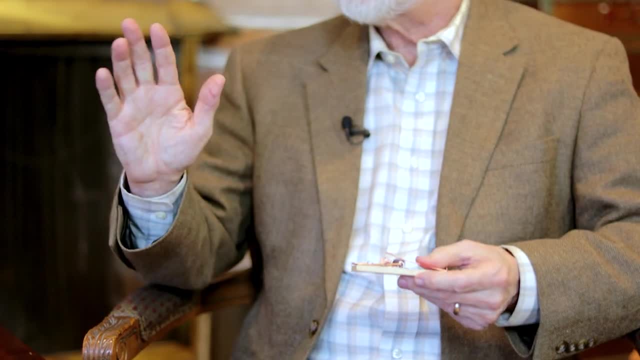 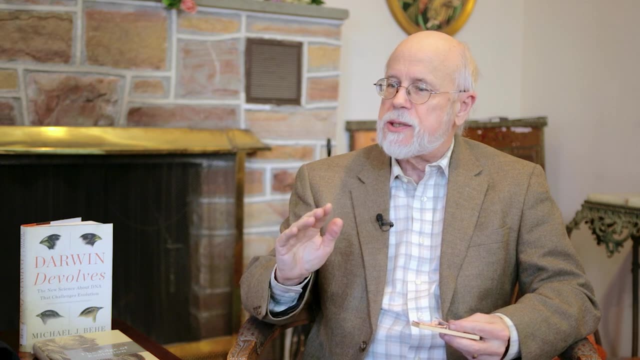 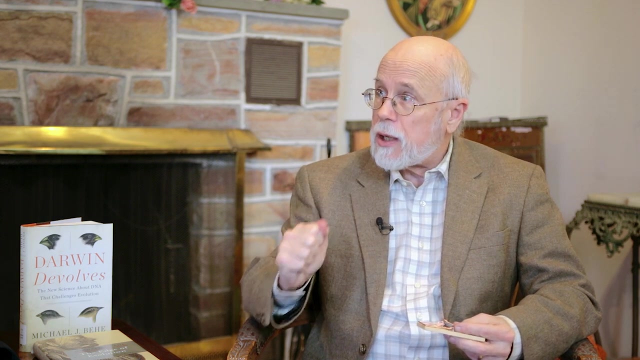 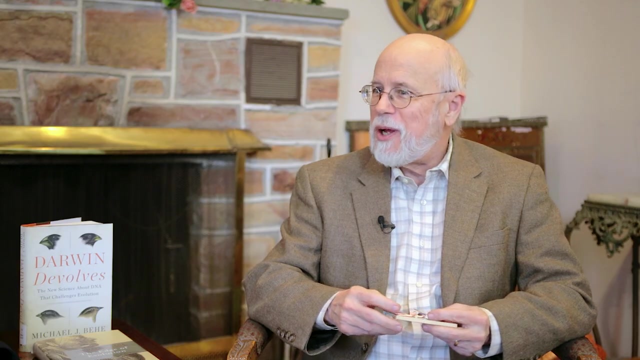 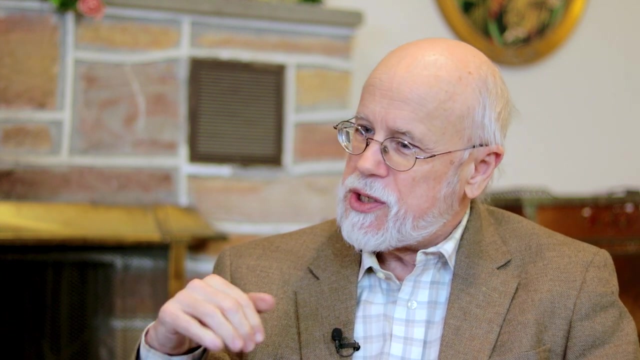 Now, the problem for Darwin's theory is that number one, the molecular foundation of life is run by machines. The cell is run by actual machines made out of molecules. People find that fantastic, but hey, that's the way it is. There are little machines that act like outboard motors that can propel cells along and other machines that carry cargo from one part of a cell to another. 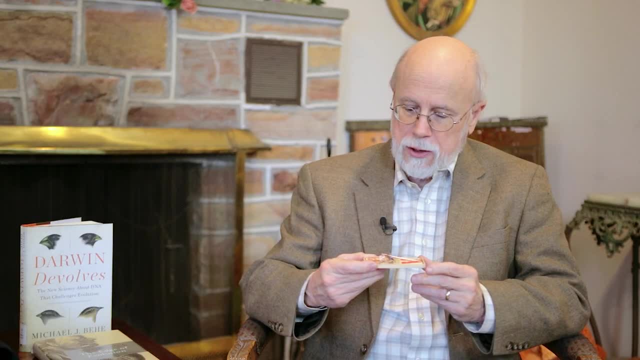 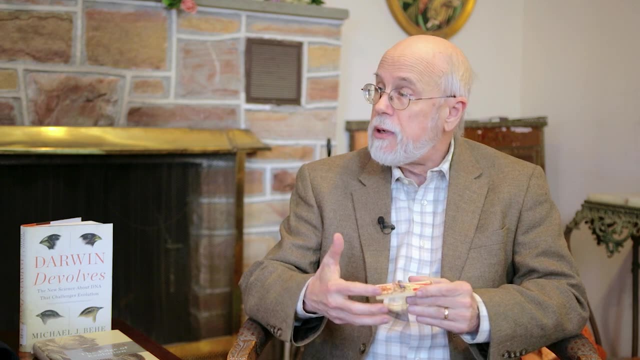 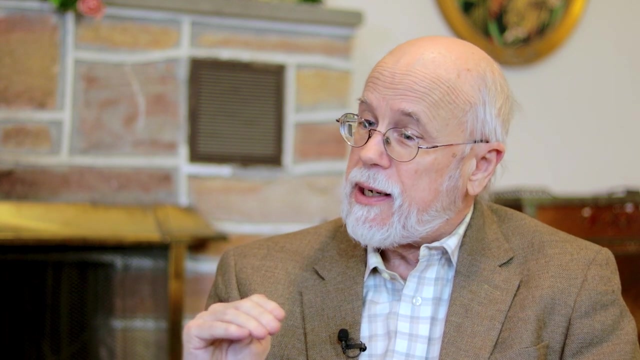 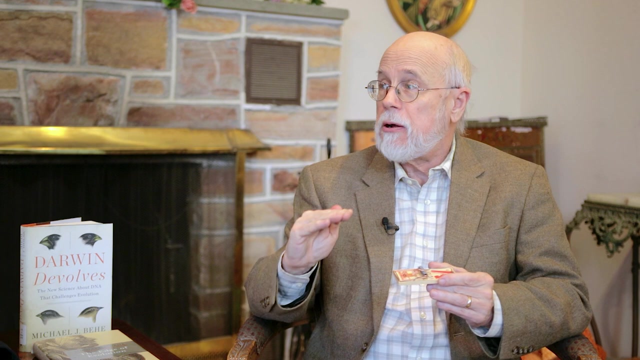 And those machines, just like pretty much any machine, including the mousetrap, have a number of different parts performing different roles and they're all needed for the machine to work. Darwin's theory of evolution requires that natural selection favor an organism that has a very small change that helps the organism do something better. 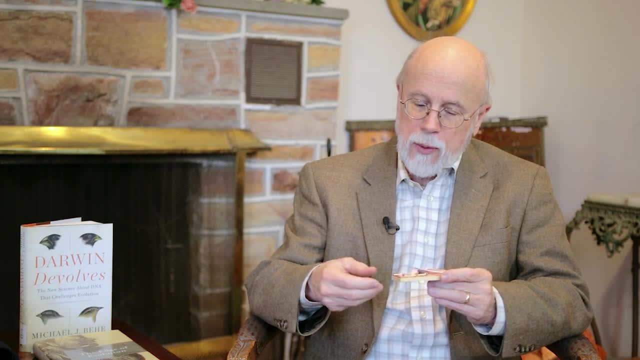 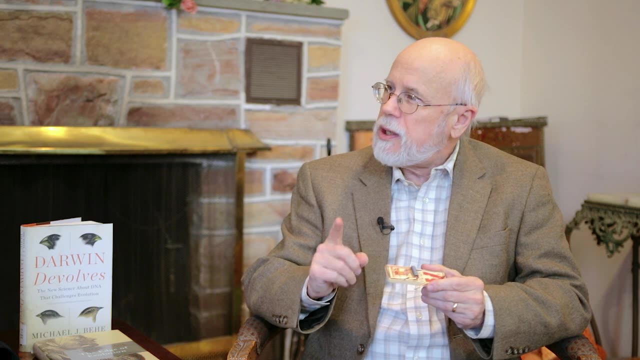 So if we're taking that view of Darwinism, we can ask: how could something like this, something like a mousetrap, be put together, one tiny step at a time, And it turns out: it's, it's. 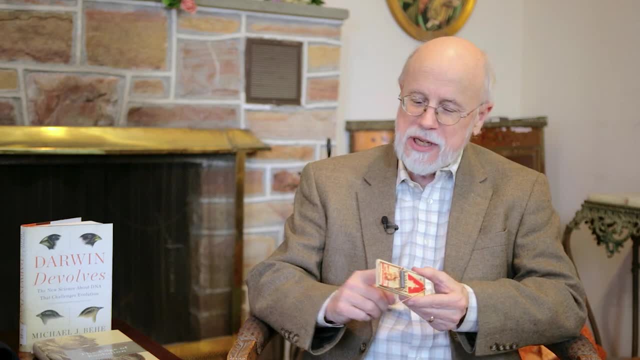 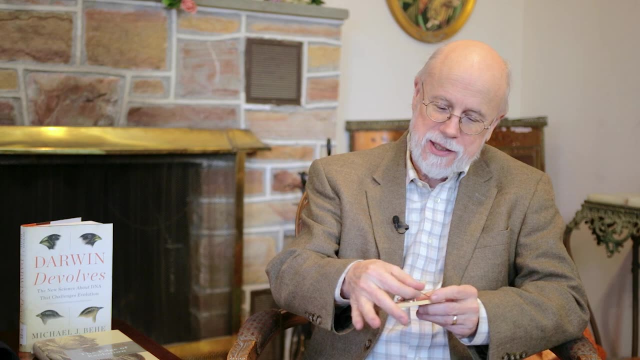 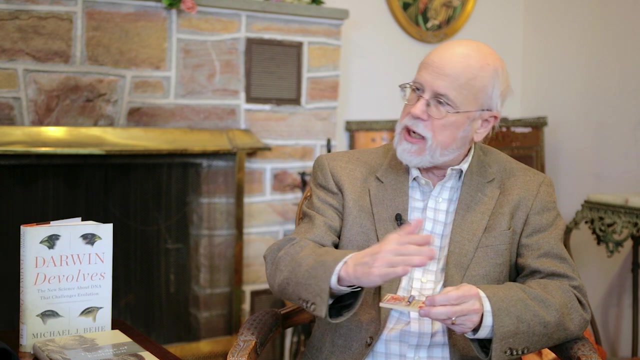 it's, it's. it's surprisingly difficult. You know, if you just had the wooden platform, just the bottom, that doesn't catch mice, If you put on, say, this holding bar, you might say, well, maybe if a mouse is running along it would trip on the platform and impale itself on the holding bar. 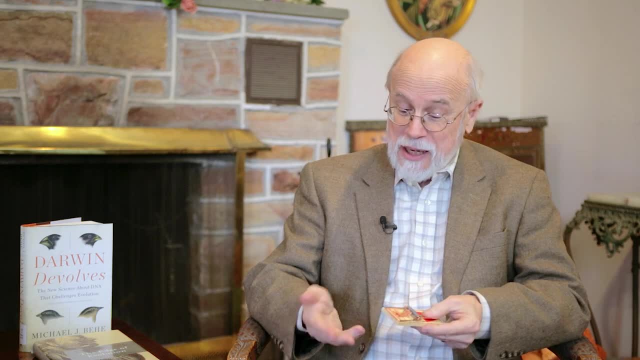 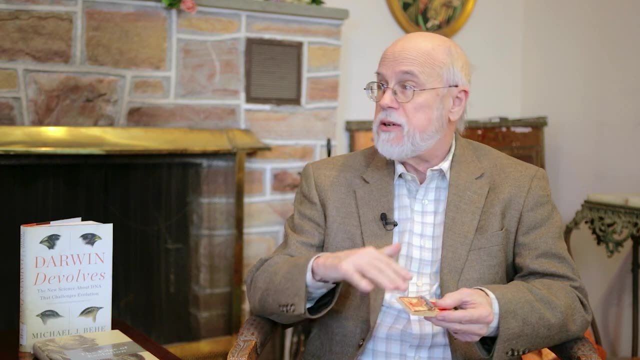 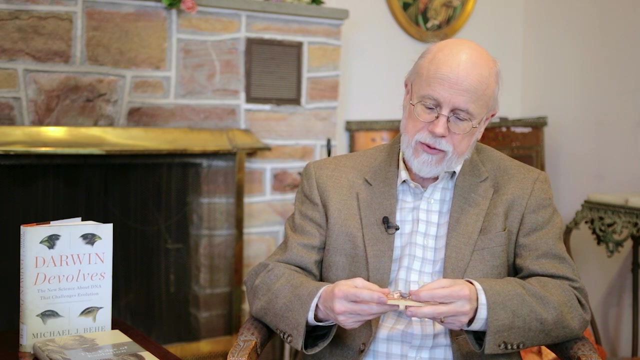 But that's kind of just silly. So this can't be made gradually. So that's a big problem for Darwin's theory, because pretty much the foundation of life, these things are all over the place And furthermore you can ask yourself: well, how do we recognize intelligence? 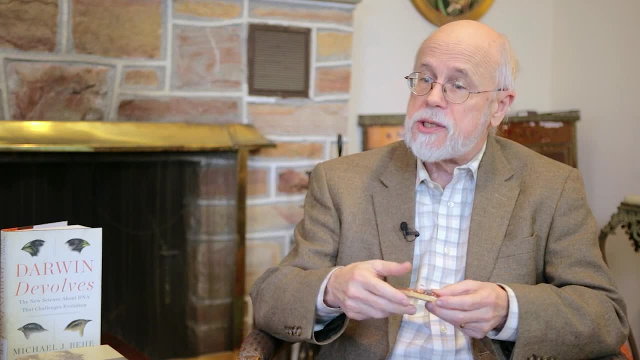 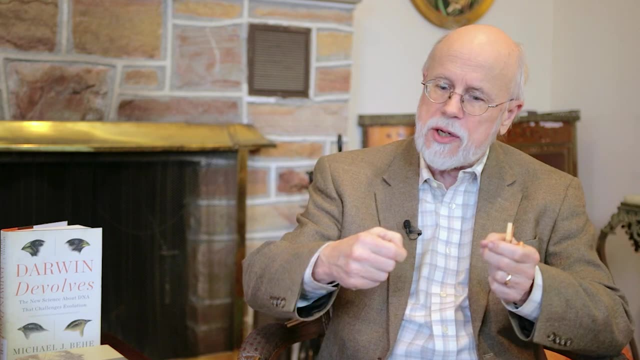 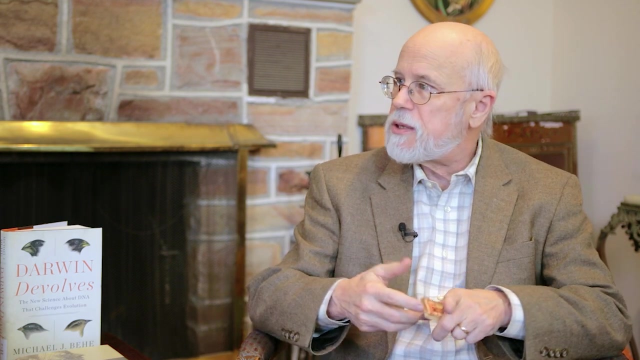 And it turns out that the way that we recognize intelligence is by what I call a purposeful arrangement of parts, And that's when different parts are put up in relationship to each other where you can see that they have a purpose. That is, the arrangement has a purpose.